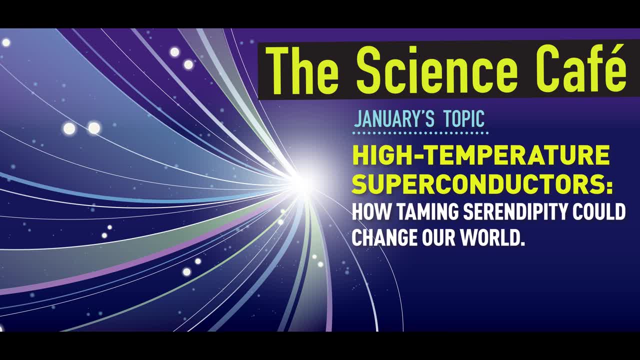 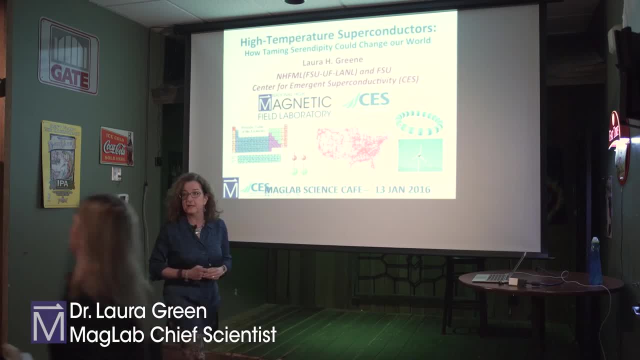 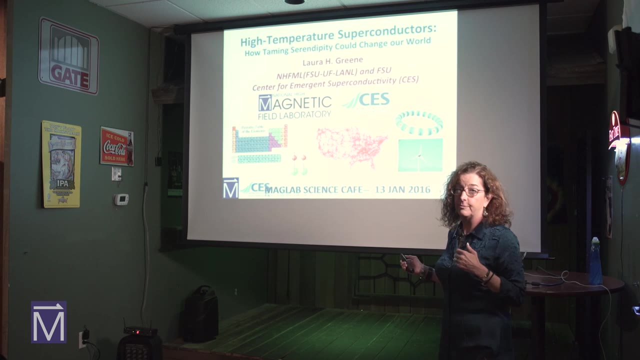 This is what we're talking about today: high-temperature superconductors, and why. if we learn how to make better superconductors, they'll transform our world. So, as Kirsten said, I'm part of the National Mag Lab Facility and FSU, and I'm also part of the Center for Emergent Superconductivity. 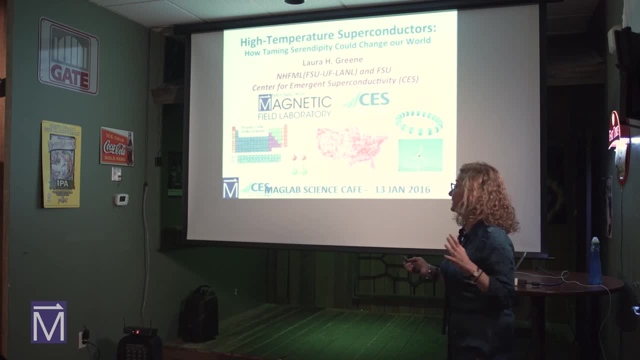 and what we worry about is using superconductivity to carry energy across with, like, the power grid, and this is what we call SMES, which is tell them to be quiet, and this is what we call SMES- superconducting magnetic energy storage- and it's basically just like a wire around in a toroid. 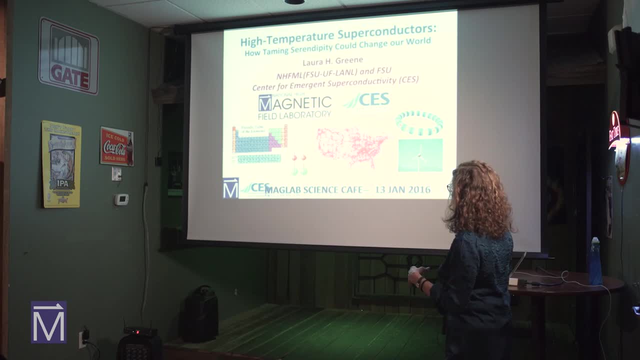 and you can save energy that way. and we also have here wind turbines. and if we could make better superconductors, going through the periodic table of the elements and understanding how the electrons move better into these materials and make better superconductors, this will transform. 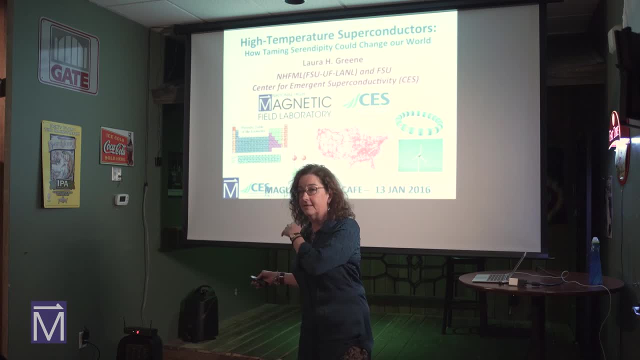 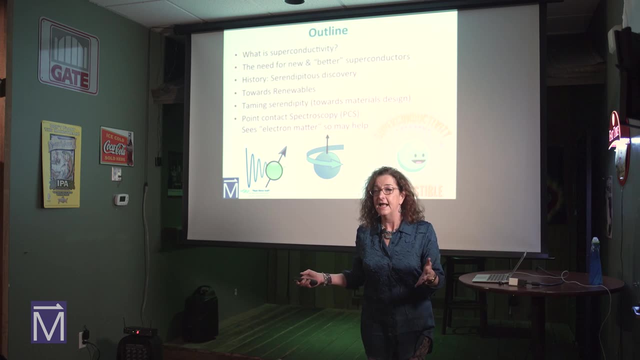 our lives. and by the time I'm done, I'll give you a quiz note and you'll understand all this. So why superconductivity? What is superconductivity? So I'll tell you what that is first, and then I'm going to tell you why better superconductors and what I mean by better. 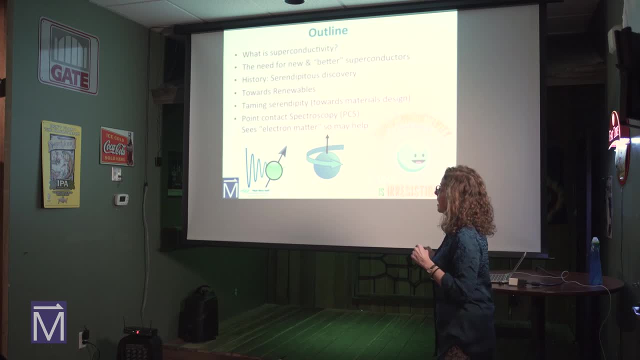 superconductors will make our lives better. I'd like to talk about the history of superconductivity and the discovery. and the discovery was not a predictive discovery. it was luck and I will stress that to you and why we still need that kind of research going on. but part of my research 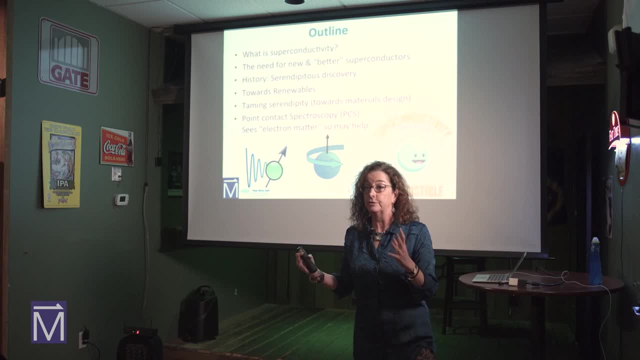 that I will continue doing here is how can we ever learn to design new superconductors, which at present is impossible. So I'll talk about some of the applications and how we're supposed to do it, and I may not get to this at the end, but how my own research will help us in this new 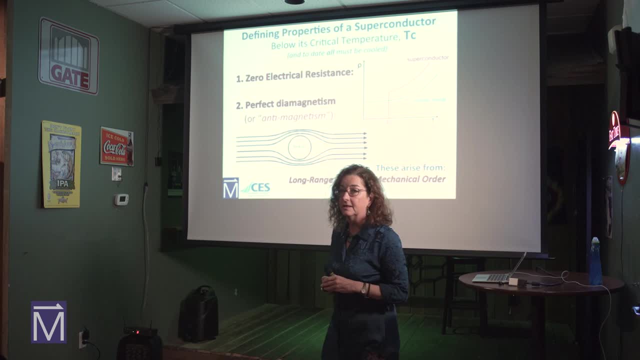 materials discovery. So what is a superconductor? A superconductor has two properties. One is that it transmits electrical energy without energy loss. that's called zero electrical resistance, okay. And the other thing is that it's a perfect anti-magnet. We call that diamagnetism. 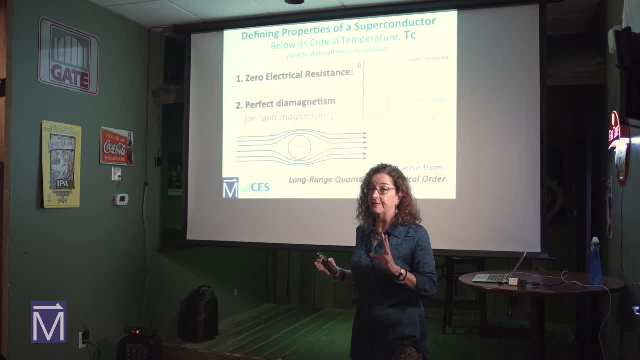 and it's very weird, and I will show you why this is very different than a regular conductor. but I'm going to show you now a normal metal. and I'm going to show you a normal metal. as you lower the temperature, the resistance gets lower. A superconductor: the resistance. 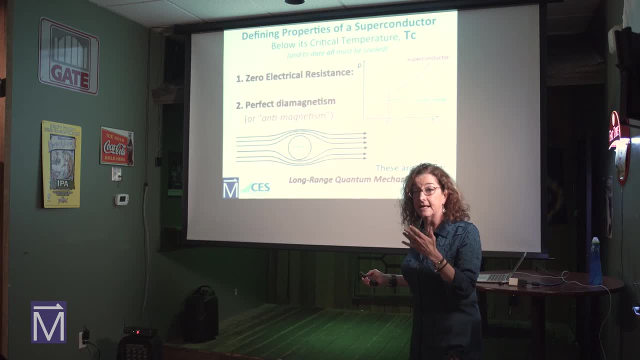 falls abruptly to zero. How strange is that. And then the other thing is anti-magnetism, which I'll talk about in the next slide or two is that if you send a magnetic field into a superconductor, it spits it out, it hates it, it absorbs any kind of magnetic field. 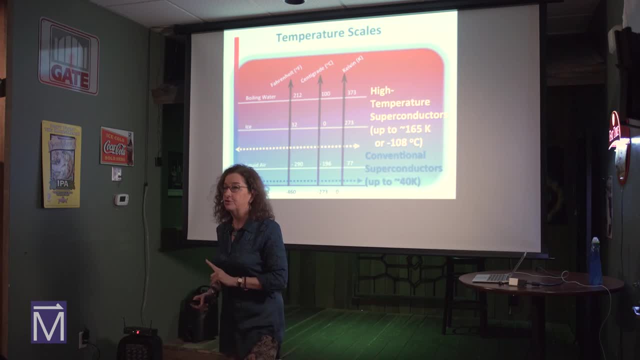 Now, no superconductor superconducts at room temperature To date. every superconductor has to be cooled and it has to be cooled at room temperature. So if you send a superconductor into a superconductor, it has to be cooled a lot. And here's some temperature scales: 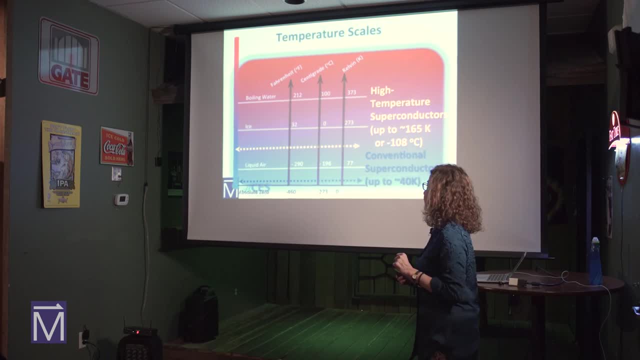 just to remind you- I know Tim and other people have given you these scales before- but what we're used to thinking of here in the United States is the Fahrenheit scale, where ice, which has been in that way lately around here, is at 32 degrees, And then, if we go down to 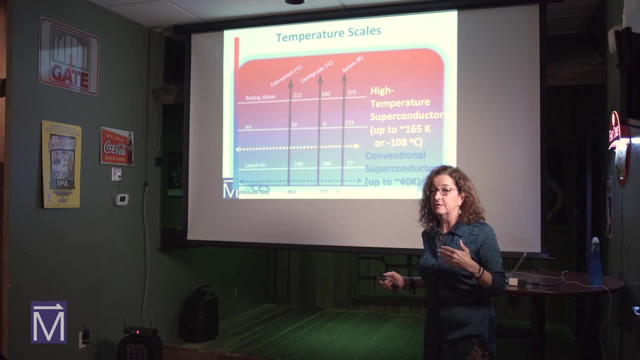 liquid air or liquid nitrogen, that's minus 390, and absolute zero is like over 450 degrees below zero, Now in low temperature. and then there's the centigrade scale. and then there's the centigrade scale which you may have heard about And unless you work in a hospital. 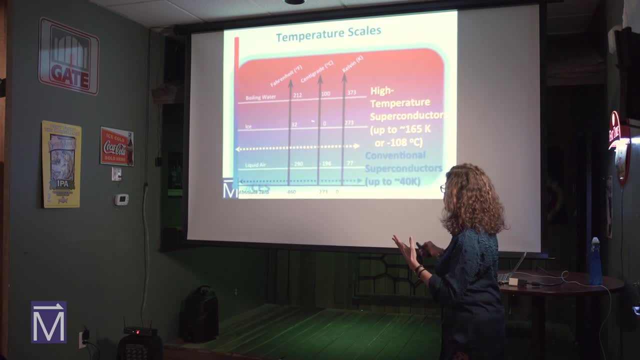 then you call it sonigrade, which I never figured out, And there zero is freezing and minus 273 is what we call absolute zero. Now, these are not what we call thermodynamic temperature scales, because if you go outside, and whether you're talking about Fahrenheit, 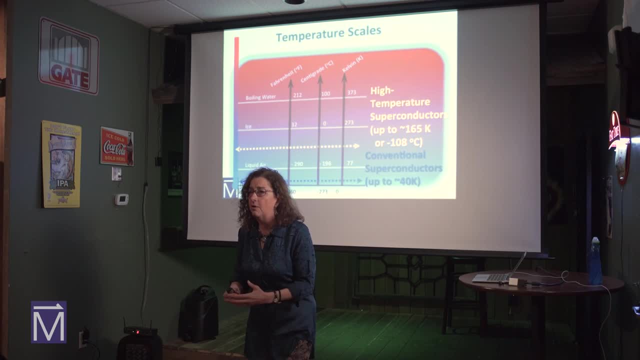 or sonigrade, and it's really cold. it's so cold, it's zero degrees outside Zero degrees, But tomorrow's going to be twice as cold. Okay, that doesn't make any sense. So what we do is we come up with a scale that you could multiply the temperatures. 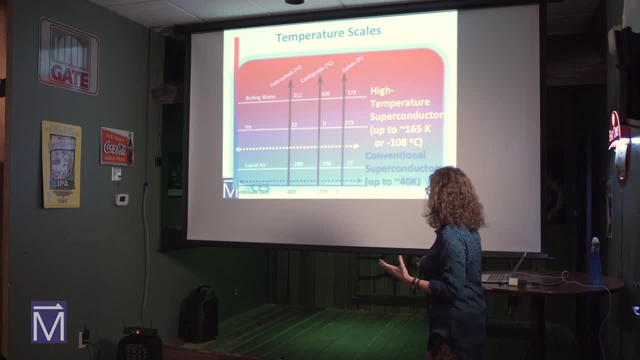 together and that's the Kelvin scale. It's thermodynamic. In that case, zero is zero Zero. if you go out in the middle of space, away from everything, you're very close to absolute zero, Not quite. We have the Big Bang, which gives us three degrees in the 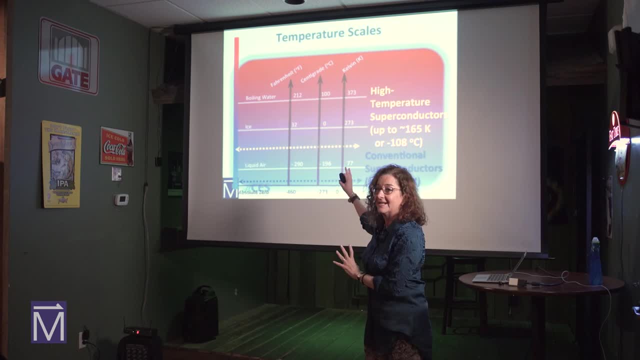 background. It did happen, I'm sorry, And that's a thermodynamic scale. Now all superconductors have to be cold, What I call the conventional superconductors had to be cooled down to very cold temperatures like four degrees to 10 degrees to 30 degrees above absolute zero. What was very exciting with 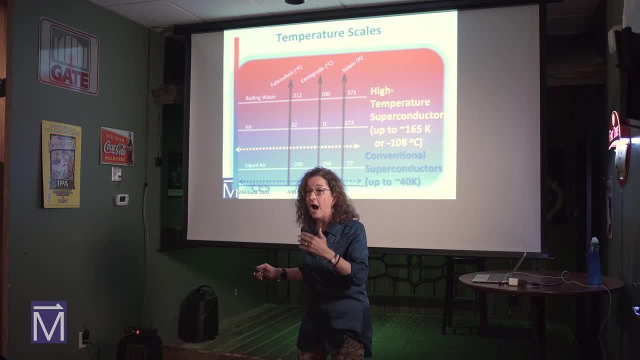 the high temperature superconductors is they could be cooled to like 100 degrees above absolute zero. Why is that important? To get to those very, very cold temperatures? it's difficult, And I'll show you some of the difficulty. You have to use something called liquid helium and it's very, very expensive and it's very 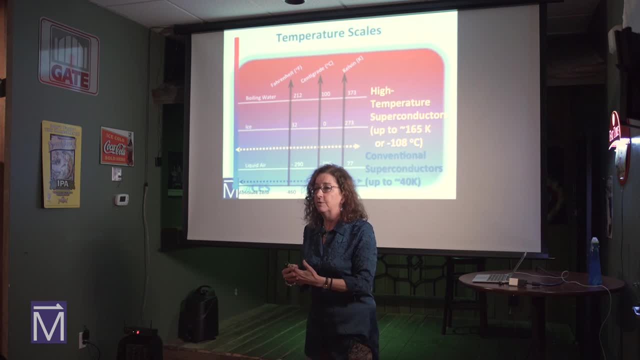 hard to use. My last university we were paying between $15 and $20 a liter and to cool down one of my cryostats it could take 50 liters. It's really expensive. Now liquid air which now the high temperature superconductors can be cooled with, it's just liquid nitrogen. 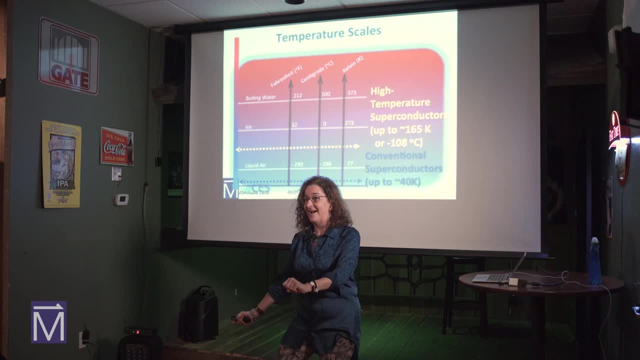 liquid air. You can pour it on the floor. I was going to bring some, but it violated some safety rules. so come visit me in the lab, Come to open house. We'll have great demos. But this is really cheap. It's like 20 cents. 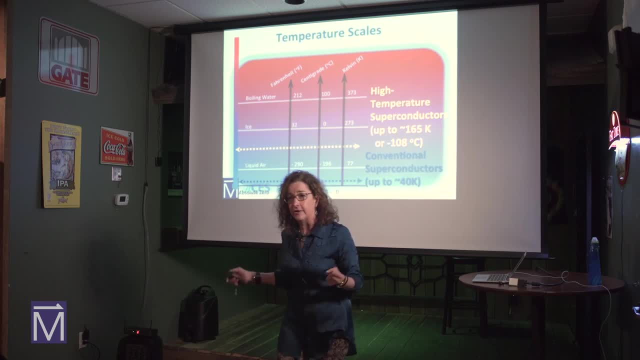 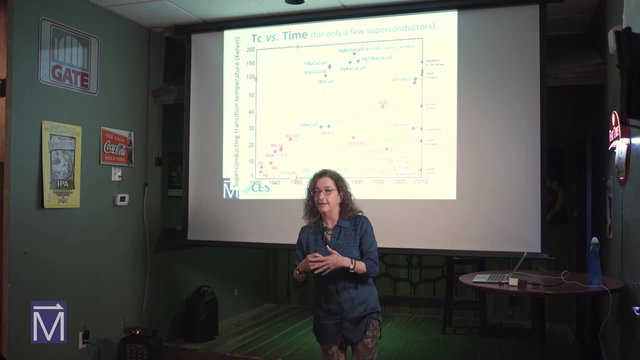 a liter, So it's cheaper than milk. I mean, it's cheaper than beer. So if we look at the history- and I'm going to talk a lot about history too, because physicists are natural philosophers- We like music, Hi, husband, We like music and history and humanities. 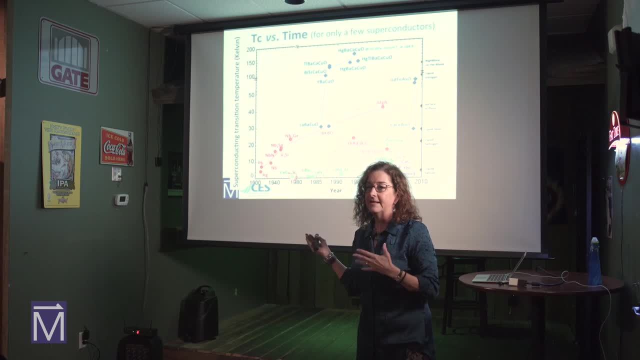 and so we'll do a lot of historical things here, And this is one of the best examples of what we're going to do here. We're going to do the many, many plots of Tc versus time. Tc is critical, temperature Above that critical. 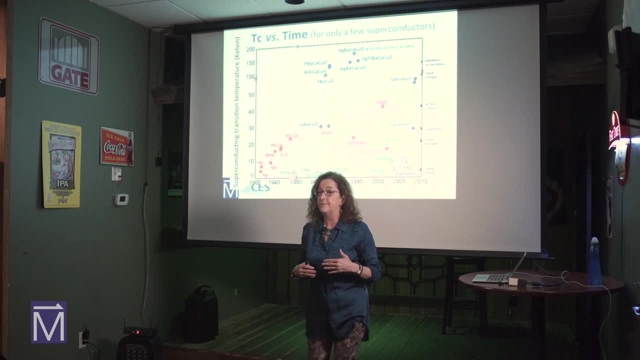 temperature. it's not a superconductor. Below that critical temperature it is a superconductor And I'll show you the camera with. onus in 1911 discovered that mercury was a superconductor And there were many discoveries and what we have here is plotting the temperature below. 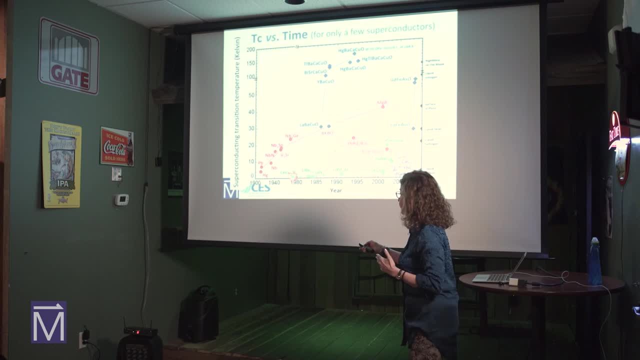 which you have to go to make something superconducting, and what year was discovered. So this is the highest Tc material discovered. That's basically the. So this is the highest Tc material discovered. So this is the second most important area in the world. So good luck with this, Thank. 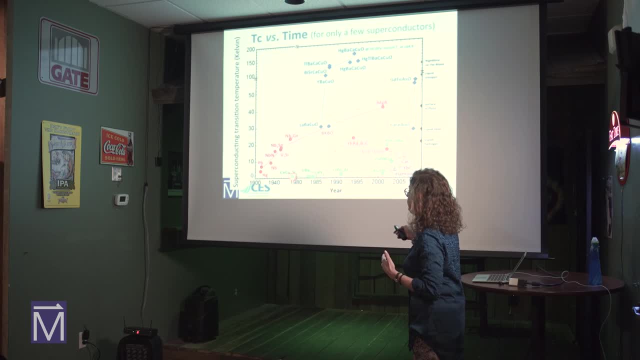 discovered in that year And it looks like what happened in 1986, a whole revolution happened And that's the revolution of high temperature superconductivity. Many of the people in this room and many of my colleagues and me- it changed my life. 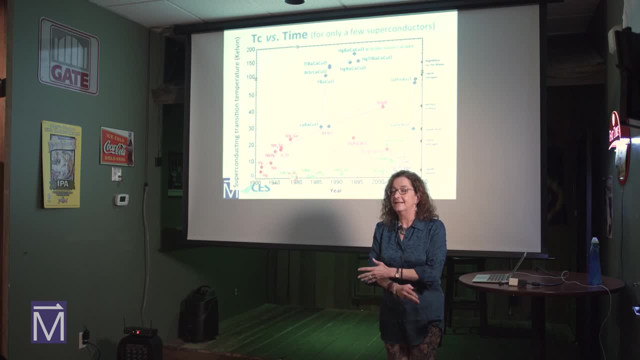 It was the most wonderful, exciting thing. We'll get a few beers and maybe I'll tell you some of the stories. It's really fantastic. But one thing I'll get across before I'm done with this talk and I'll tell you first, right now. 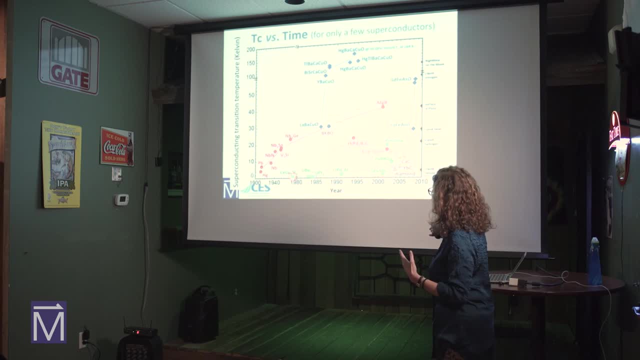 and I'll say it again later- is that there are many superconductors that aren't on this red line. here. This red line, and everything is red, is what we call a conventional superconductor, And that's one of the two problems in what we call correlated electron physics. 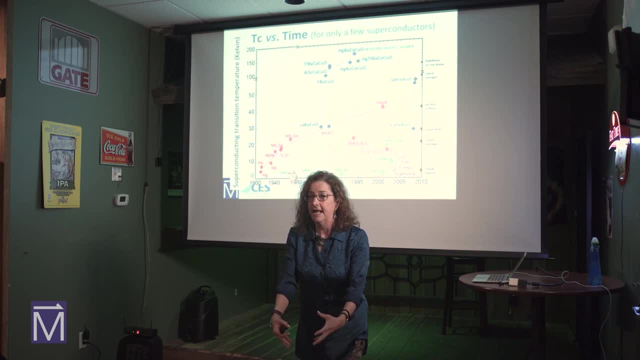 That means you've got to use quantum mechanics to describe it. And, as Richard Feynman says, no one understands quantum mechanics, One just gets used to it. And what happens- and I will show you- is that these electrons At actually pretty high temperatures, 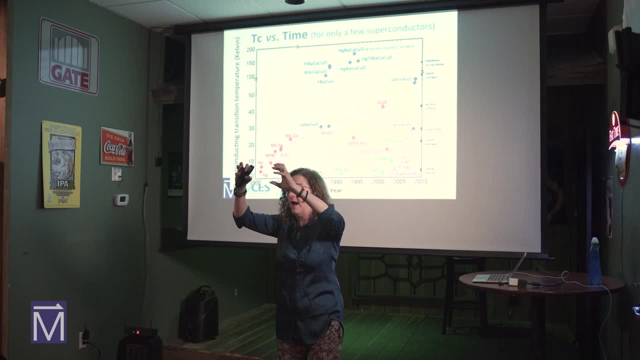 start skipping together, doing things that we don't know why, and they correlate over pretty long distances And that's what's understood. But what we do understand is that when we go below this critical temperature and the things are superconducting- that's understood. 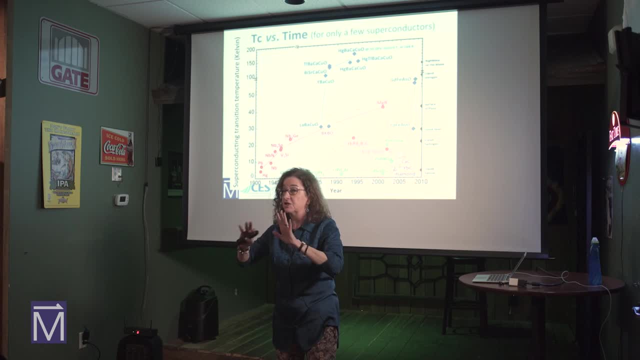 We even have mean field equations to describe the properties, the transport, the optical. We can do that, But exactly Exactly. We can describe the properties, but exactly why they superconduct Everything. that's not one of these red dots here. 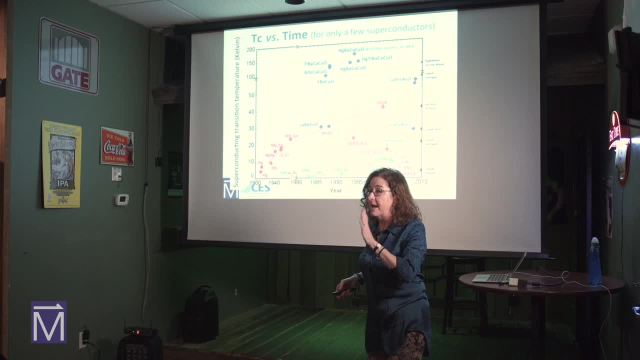 we can't explain, And let me tell you that I have many, many families of superconductors I haven't put on here. So all of the high temperature superconductors and many of these other correlated electron superconductors, we don't know how they work. 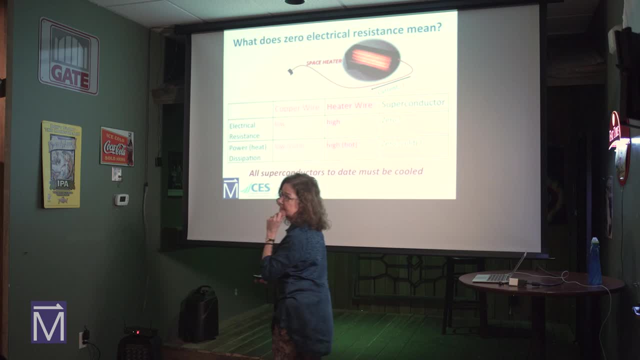 And that's the focus of my work. Now, what does zero electrical resistance mean? Let's consider: this is a space heater which I've like understand that some of you have actually seen before in this room. I came from Illinois, so we know space heaters. 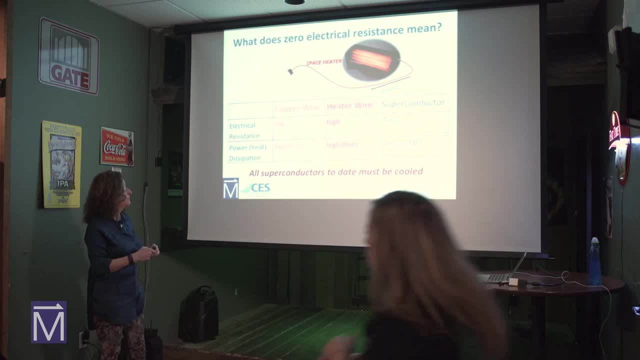 So if everything is working correctly in your space heater, when you plug it into the wall, the current goes through the copper wire And the coils. if you unplug it and let it cool down and make sure it's unplugged, the coils are hard and black and stiff. 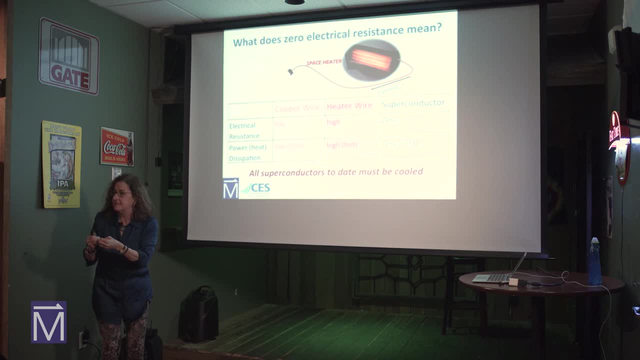 This is a material that's designed to be very resistive. So when the same, when the, The current goes through the low resistance copper wire, There's not much loss, there's not much resistance. In physics, the power loss goes as I squared R. 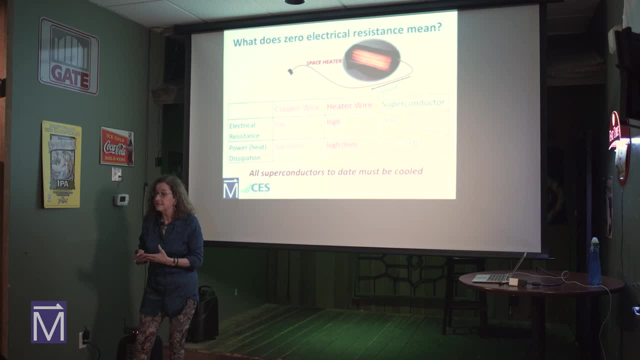 It's proportional to the resistance. If it's a high resistance, there's a lot of power dissipation, it gets hot And that hard crinkly wire it's like the electrons can't get through. it's like rubbing your hands together, right. 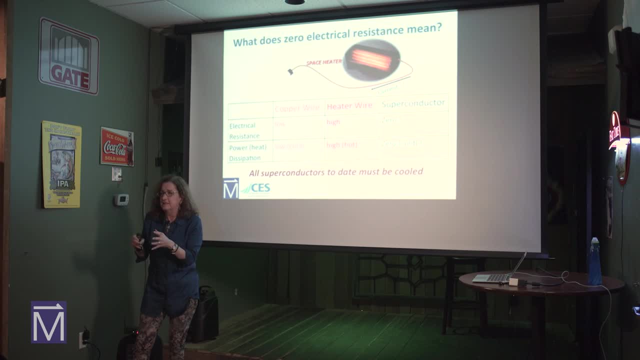 Instead of rubbing on something soft, smooth And it really feels this resistance. Now, a copper wire is low resistance, so there's little heat dissipation. The heater wires are designed to have high resistance, so they get very hot. A superconductor if everything's working. 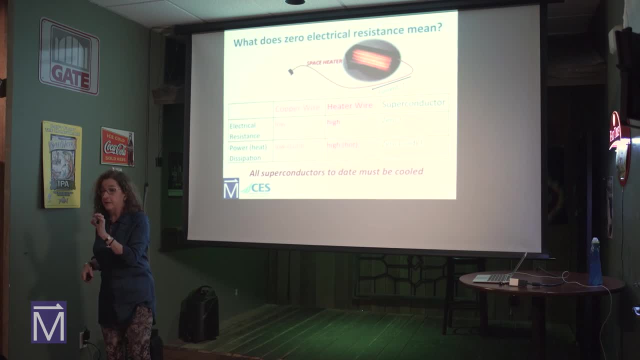 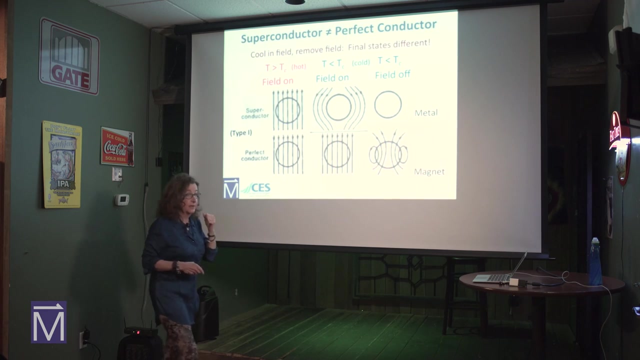 has zero electrical resistance. So if you have a light bulb here and a battery in Southern California and it's connected by superconducting wires, that light bulb will light. No energy loss, no power dissipation, So Pretty cool. 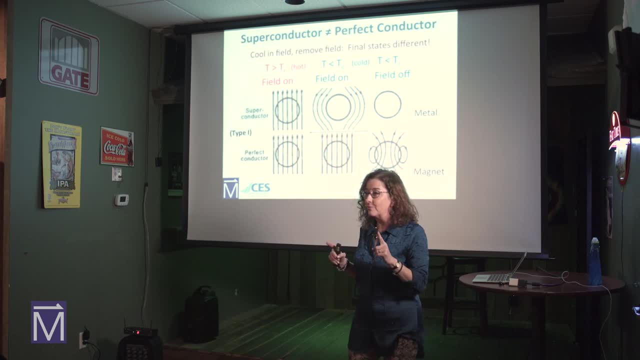 But it's not just a perfect conductor. There's something really creepy in there. It's a superconductor, which is distinctly different than a perfect conductor, And what this diagram here is to show you the difference between a perfect conductor and a superconductor. 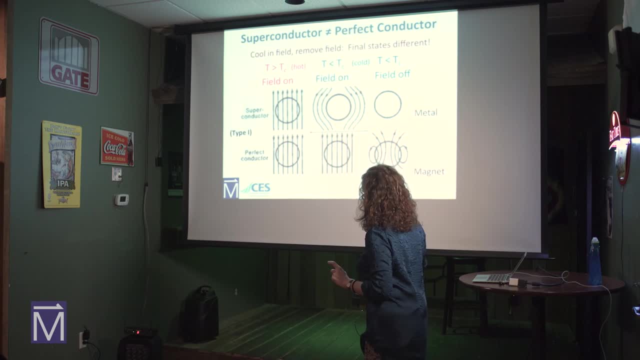 Now this is an example of a perfect conductor. First you put a magnetic field on it at high temperature, above its critical temperature, when it's conducting like a regular piece of metal. And that's the magnetic field. Let's say we lower the temperature. 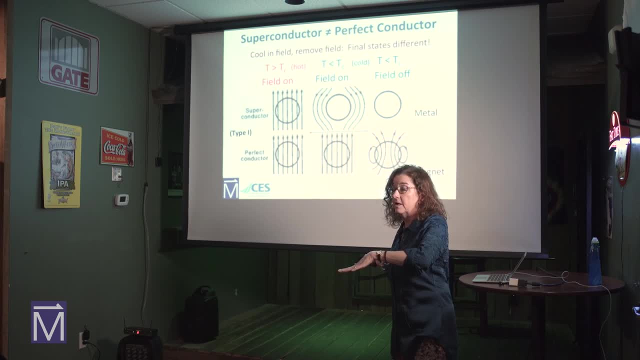 thunk below the perfect conductor's critical temperature. So now it's a classically really great conductor. Mr Maxwell in his equations told us that if something is a perfect conductor, those magnetic field lines get stuck And you can't move them out. 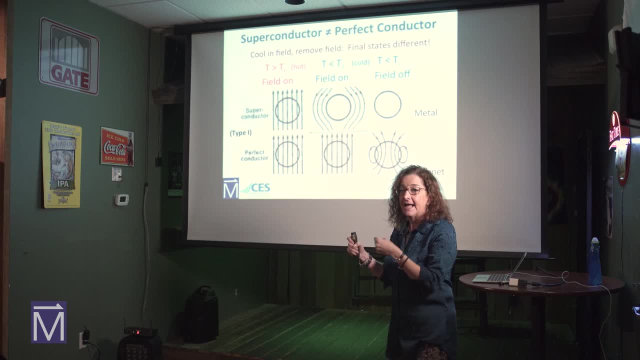 She can drop off some food, OK. And in fact, if you have a superconductor, if you stay at that low temperature and you take off the external field, those field lines are stuck and the final state is: in fact. 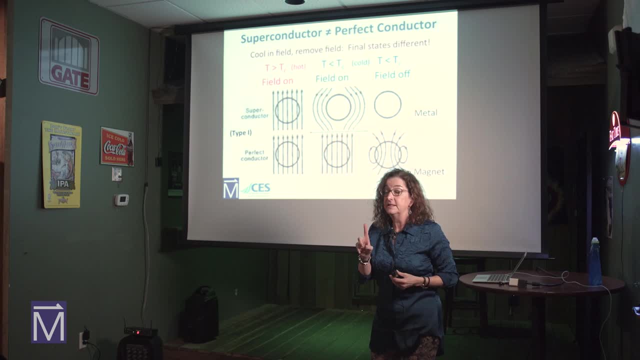 looks like a little magnet, A superconductor, does something completely different. This was discovered by someone named Meissner and a student named Aschenfeld, But we don't call it the Meissner-Aschenfeld effect. we call it the Meissner effect. 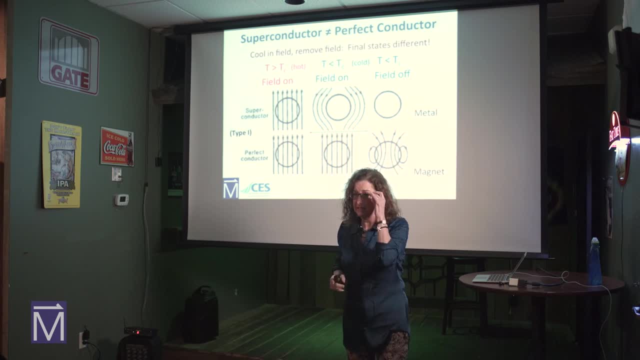 So if you know any graduate students, tell them to get their PhD and get out so they can start getting credit. Anyhow, The Meissner effect that was discovered in the 1920s, if you put a field in the superconductor. above its superconducting transition temperature and then you lower it to below its critical temperature, the field lines aren't stuck, They're spit out, Literally thrown out, And the result is, when you take the magnetic field off, you don't have a magnet. 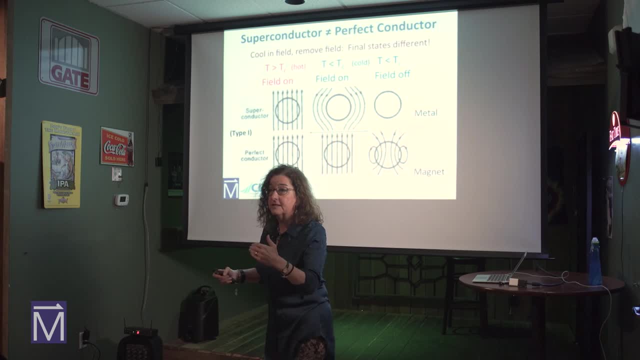 So you take two materials, a perfect conductor and a superconductor, and you put them through the same processes and your final state is different. That's a proof that a superconductor is fundamentally different than a perfect conductor, And it's this quantum mechanical Meissner effect. 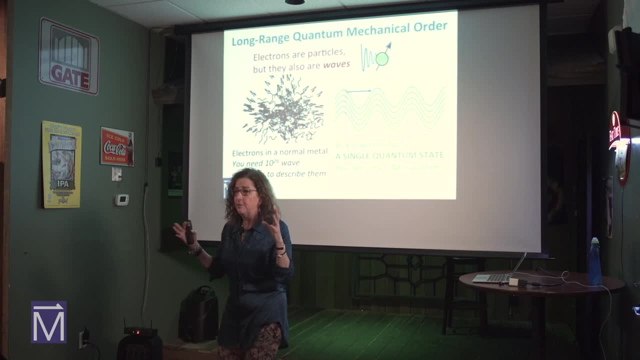 This quantum mechanical Meissner effect and I'd like to talk about this, but I won't have a lot of time in this talk. It proves that there's long range quantum mechanical order. So inside of a superconductor, the quantum mechanical order. 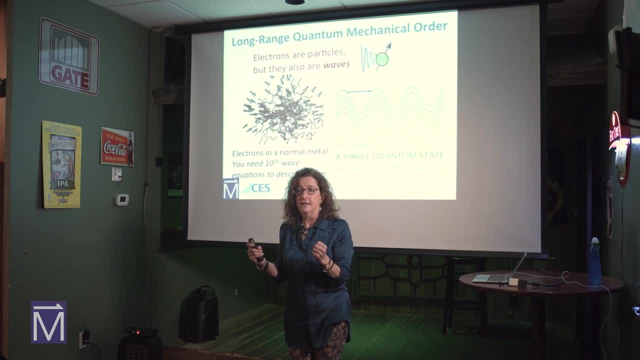 is that those electrons are really holding hands over very long distances. The typical length scale in a metal is like an angstrom In a superconductor. it could be microns, It could be 10 to the third to 10 to the five times longer. 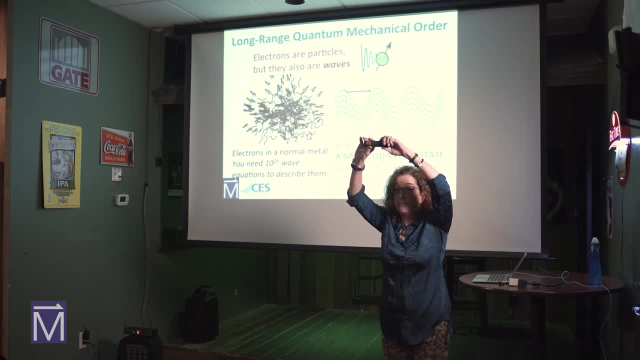 And what happens is, instead of like if this pointer were a piece of metal, here each electron is going to act like a little wave. You may have heard that, And they're unrelated. If this were a superconductor, it would be a superconductor, and I lowered it down. 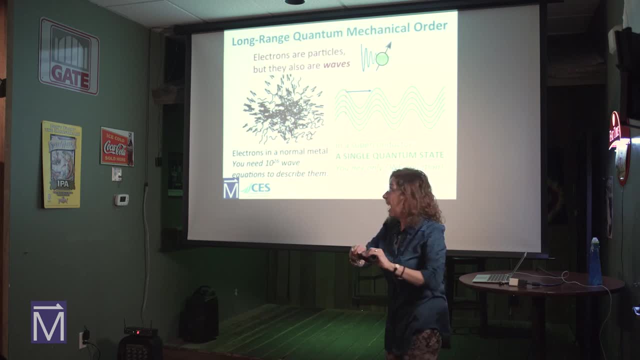 to below its superconducting transition temperature. I don't have all these little electrons acting like little waves. They all form into one wave. That's the BCS theory of superconductivity. I don't need 10 to the 26 waves to describe it. 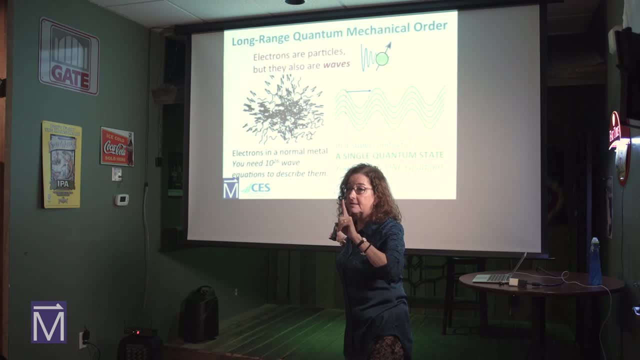 I need one wave. They fall into a single quantum mechanical state, macroscopic, And I'll show you some examples coming up. But it is really cool, right? I mean, All of a sudden you have quantum mechanics on as large a scale as you want. 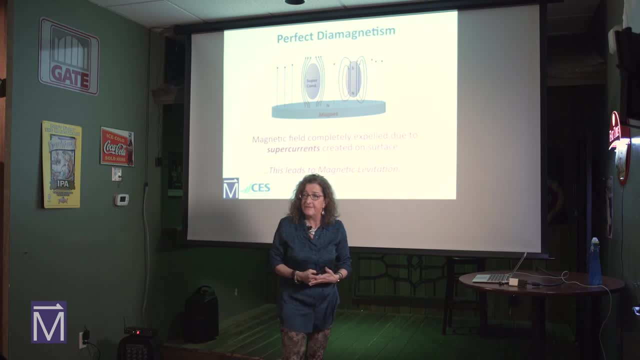 Now this perfect diamagnetism works because, in fact, the electrons move without any resistance. And a cartoon- And, by the way, I want to tell you that I use a lot of analogies in these talks And, just to warn the experts, all analogies break down. 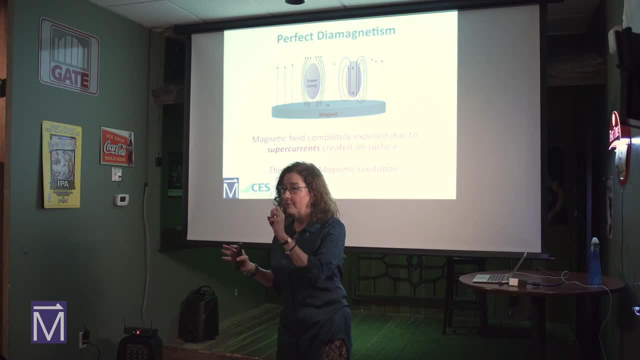 if you push them too far. So, for instance, maybe you've heard of the Bohr model of the atom where you've got these little electrons like planets around the sun. Completely wrong, OK, But we teach it and we use it because it. 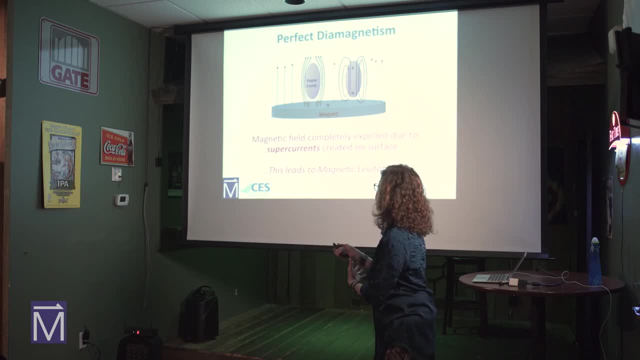 helps us understand it. So I'm just warning you for some of the experts. In any case, if you put a superconductor on top of a magnet, as I mentioned to you, the field gets thrown out And that's the perfect diamagnetism. 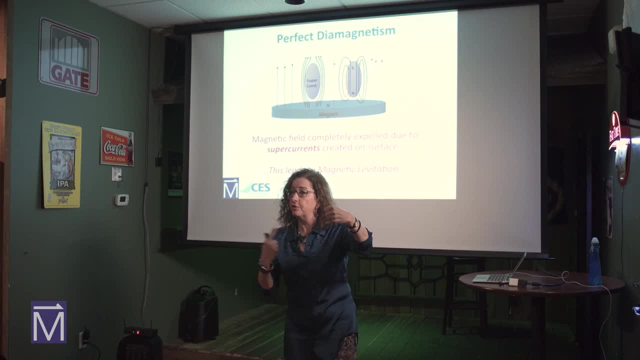 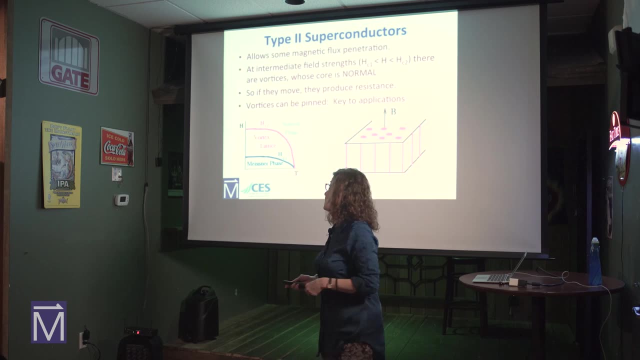 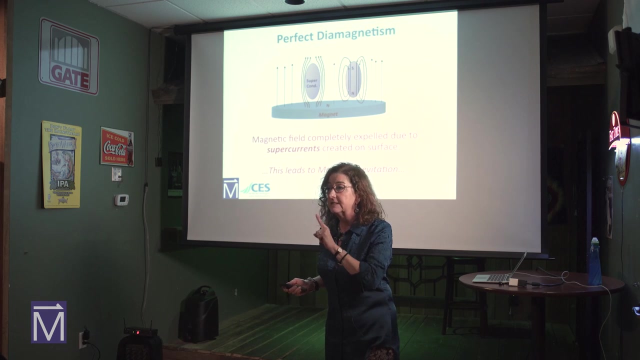 What happens is that the electrons start moving around the surface and making a magnetic field that points in the opposite direction And that causes superconductors to flow, And I'll show you that. But before I show you that, I want to show you something that's very interesting, which? 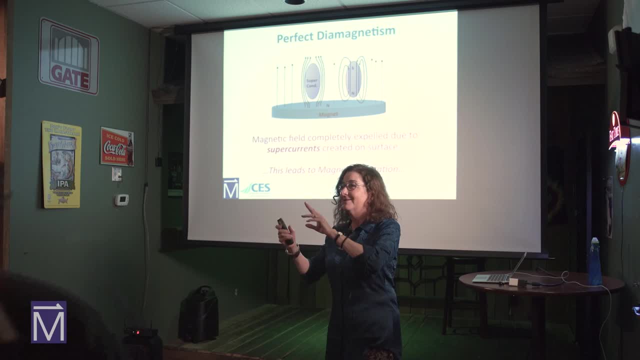 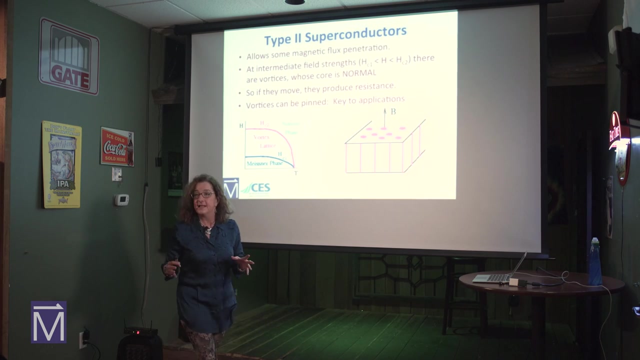 is that there's two kinds of superconductors. There's type I superconductors and type II superconductors. I bet that surprised you. OK, so it turns out that type II superconductors are good superconductors. They're the ones that are practical. And they do expel magnetic fields. But because of some intrinsic length scales, if you put them in a large enough field you don't necessarily kill all the superconductivity. You can actually have the magnetic field penetrate in little places And it causes vortices of supercurrent around there. 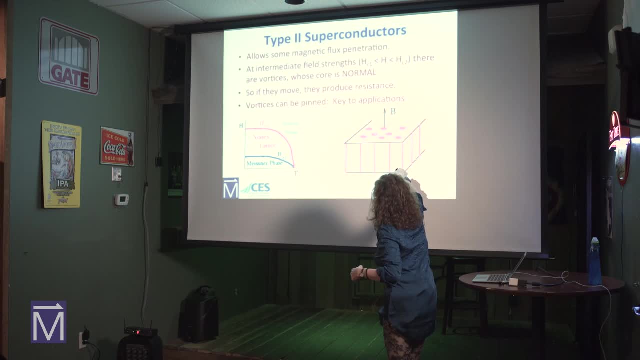 So these areas here around this vortex, around this magnetic field line that's penetrating the surface, you have supercurrents running around Now. this is very important to understand. There's one point here, Inside of that vortex, where the magnetic field goes through. 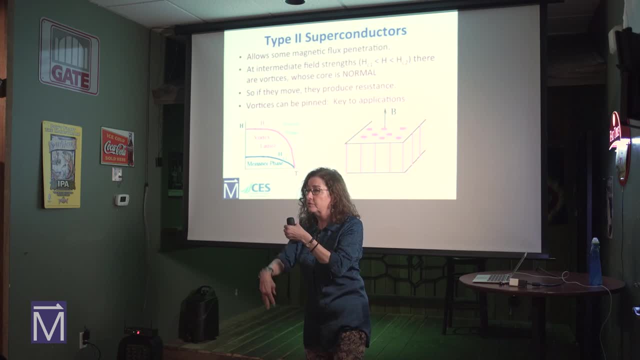 it's not superconducting. Those pink lines aren't superconducting. So if that vortex is free to move, it's going to move the inside of it, which is non-superconducting, So it's going to dissipate energy. 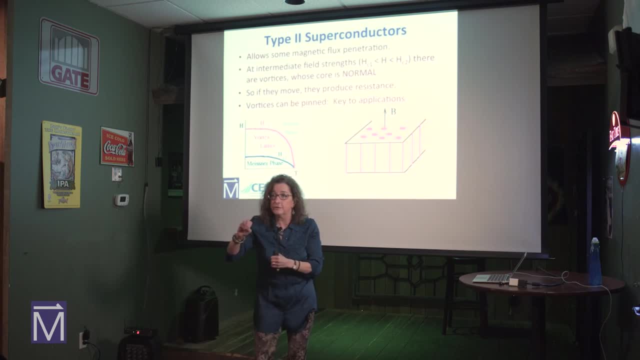 So a key understanding: in these type II superconductors, the ones that can maintain high fields, that are practical, you have to figure out a way. You have to figure out a way to pin those vortices. So that will lead us to something here. 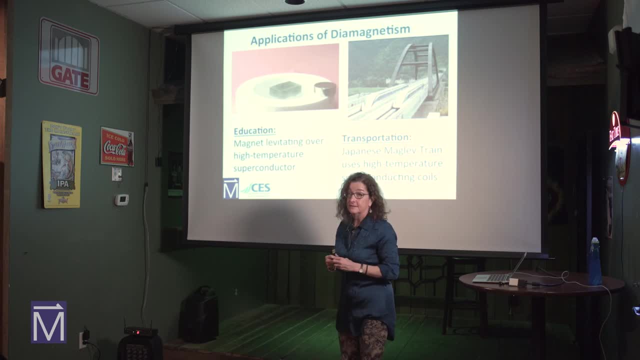 which is, if you want to make something, levitate superconductors work, great. So I have an example here And I do have the demonstration somewhere, but I'll just show you here. Here's an example. Maybe you've done this yourself. 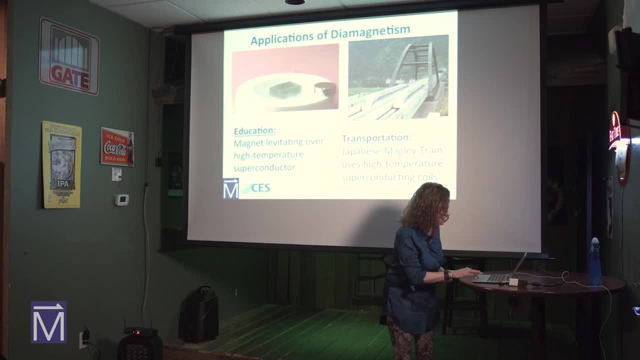 Oh sorry, I hit the wrong button here. I have to go back to here. Nobody's perfect, So come back, Come back, Come back. So this is a high-temperature superconductor that's immersed in a little bowl of liquid nitrogen. 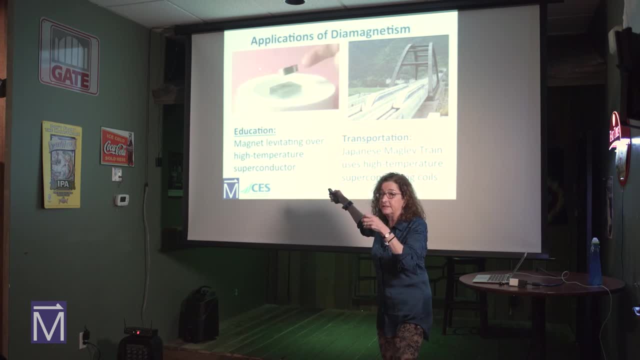 And this is a very strong magnet, And look how well that's holding on there. That's holding on so strongly because it has vortices that are pinned in there. Now, if you try to float two magnets, two permanent magnets, on top of each other, you can't do it. 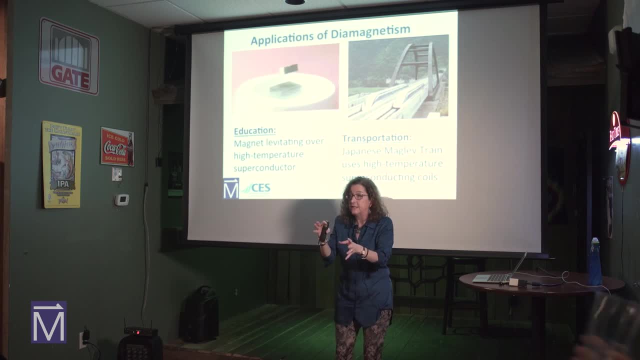 without making some special braces or doing some other special things, Because in fact two permanent magnets are unstable. It's called Harsha's theorem. So if you want to make something like a levitated train, superconductors are a good idea. 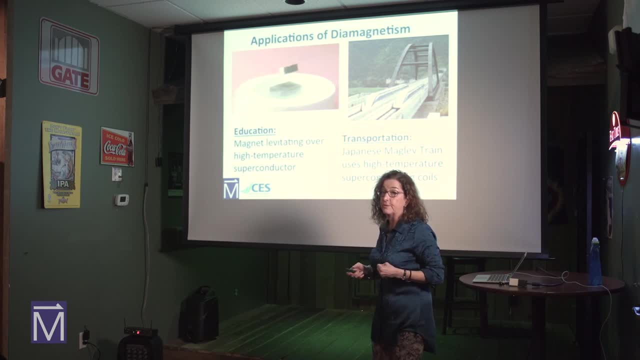 In fact, this is an example of a high-temperature, superconducting maglev train in Japan And it's a prototype. Now I've been on the maglev in Shanghai, which is really cool, But it's not superconducting. 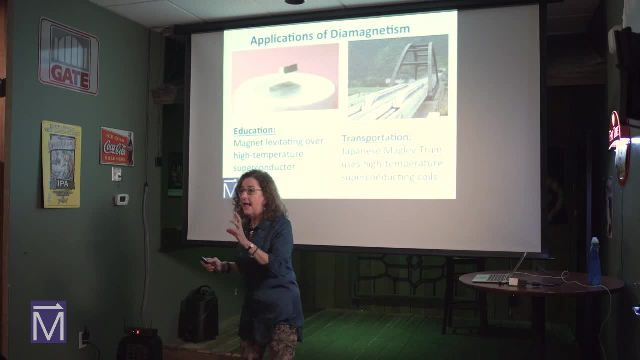 But I also want to point out one other thing is that many of the applications I'm going to show you have been around since the 60s And in fact the Japanese had a superconducting maglev train made out of not high-temperature superconductors. 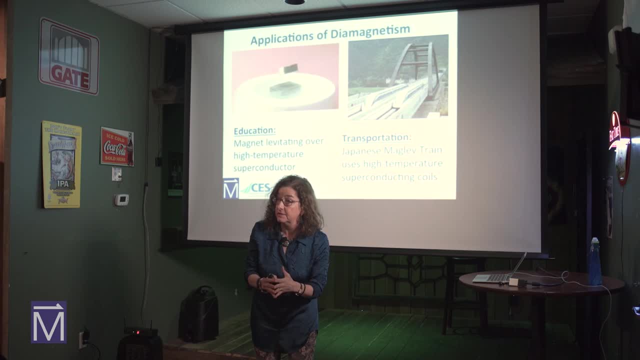 because they didn't exist then out of conventional superconductors, one that I'll introduce you to in a few slides. It went about a kilometer, And my Japanese colleagues were very proud of saying that it went just long enough to take our funding agents for a ride. 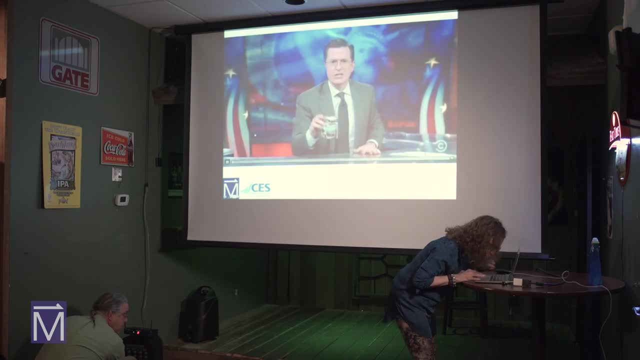 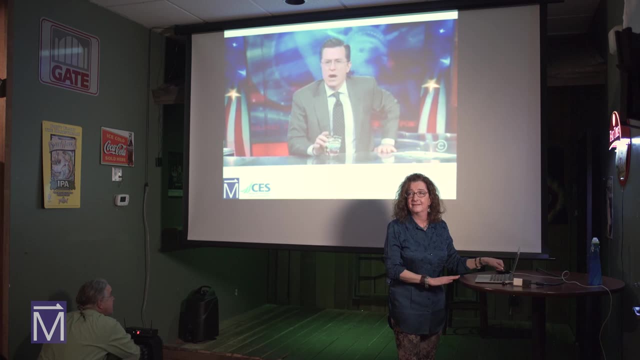 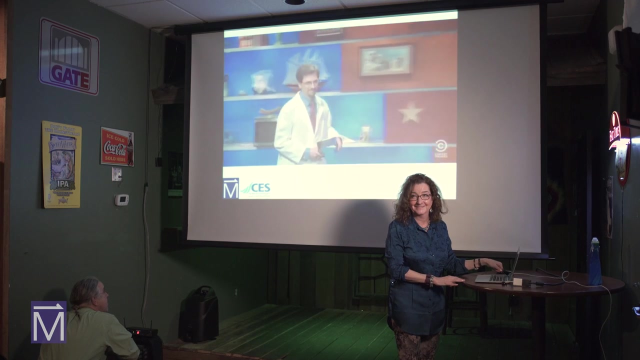 And so we're going to have a look at the results. Ladies and gentlemen, are you ready? Then please welcome from the physics department at Ithaca College, Dr Matthew C Sullivan and the quantum levitator. Thank you so much for joining me.